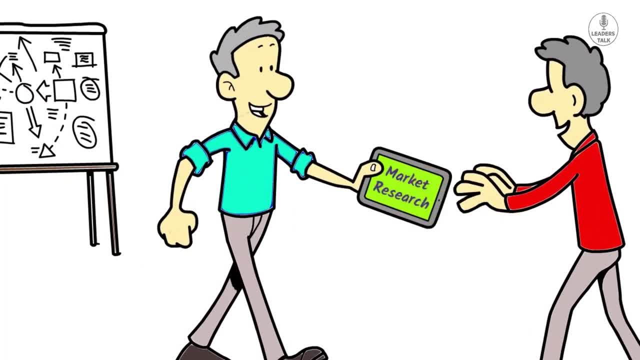 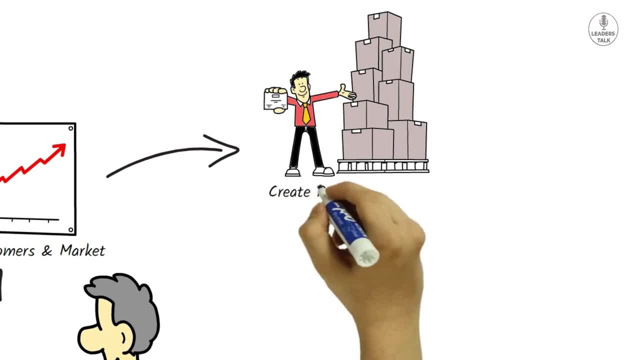 Market research is a crucial element for any successful business. It is the process of gathering information about potential customers and the market in which a business operates. This information is then used to create products and services that meet the needs of their target audience. Market research helps businesses make informed decisions, resulting in higher sales. 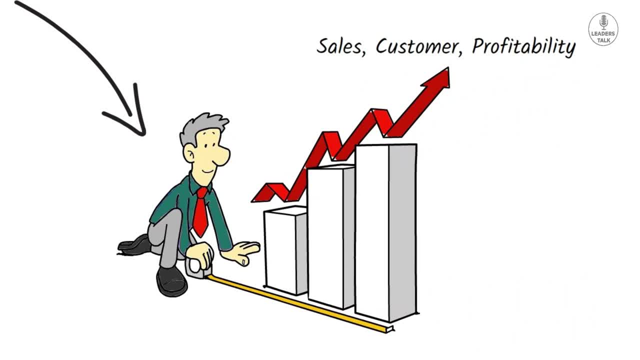 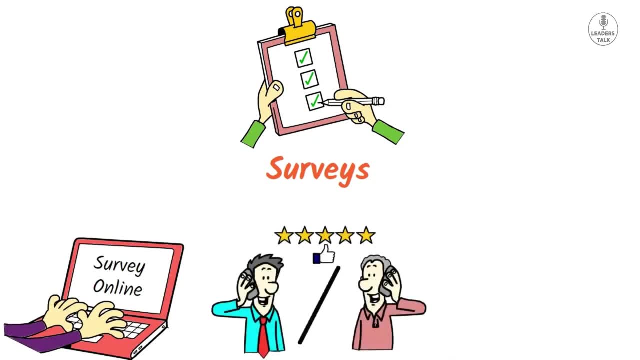 increased customer loyalty and improved profitability. There are many different types of market research that businesses can undertake. One of the most common methods is surveys. Surveys can be conducted online, over the phone or in person. They can be used to gather information about customer preferences, buying habits and satisfaction with products. 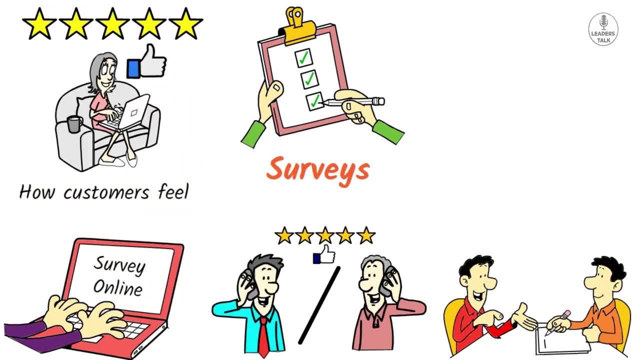 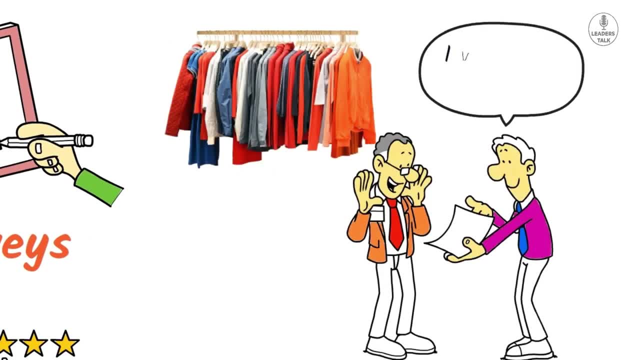 and services. Surveys can provide businesses with information about how customers feel about their products or services and what they would like to see improved. For example, a clothing retailer may conduct a survey to find out what types of clothing customers are looking for, what colors and styles they prefer and what price points they are willing to pay. 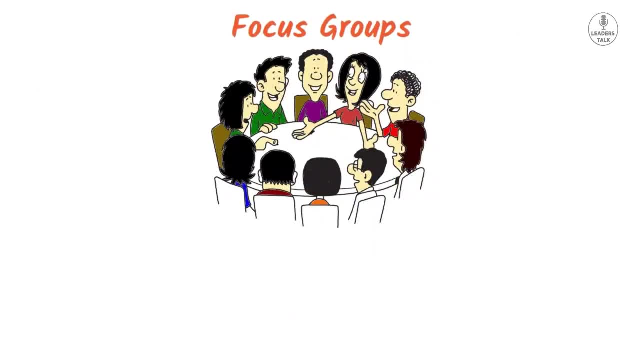 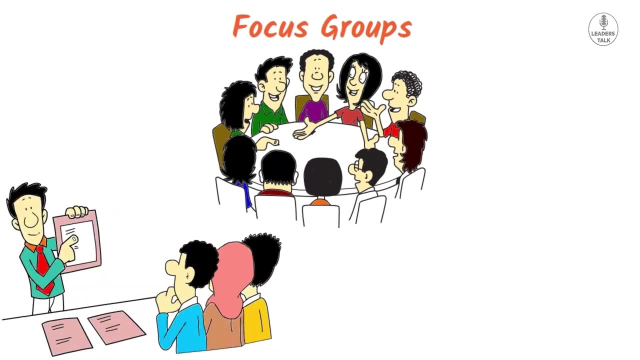 Focus groups are another type of market research. They are sometimes used to collect information about the market. Focus groups are small groups of people who are brought together to discuss a particular product or service. Focus groups can provide valuable insights into consumer behavior and help businesses identify areas for improvement. Focus groups can be used to test new products or 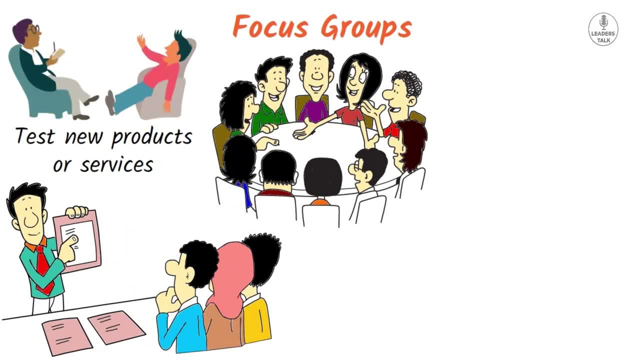 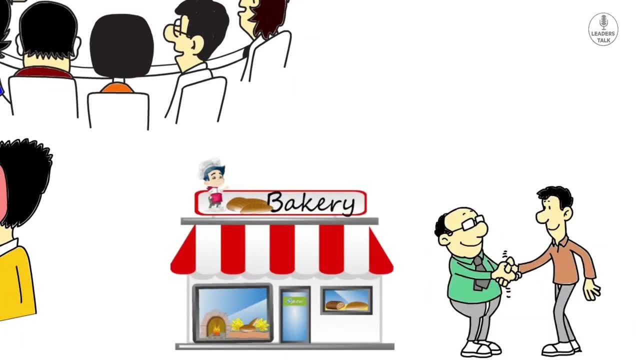 services, get feedback on existing products and understand how customers make purchasing decisions. For example, a fast food chain may conduct a focus group to get feedback on a new menu item before it is launched to the public. The focus group participants can provide feedback on the 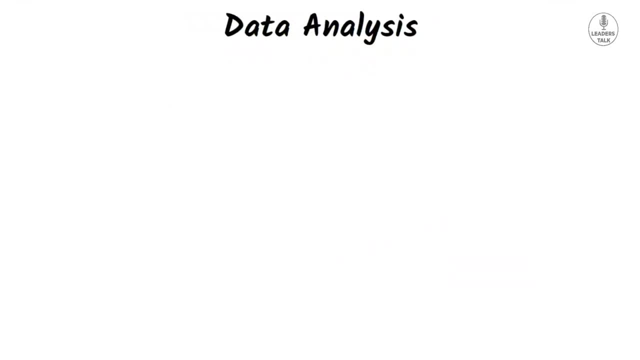 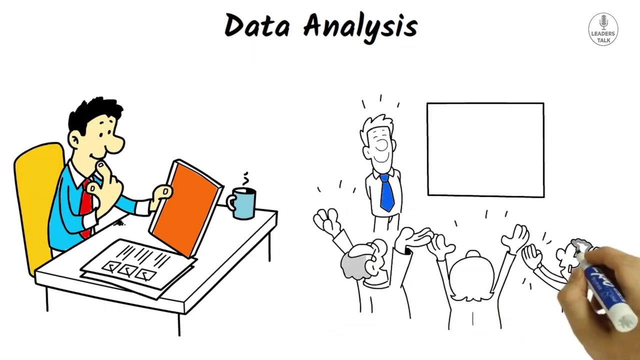 taste, price and overall appeal of the menu. Data analysis is also an important part of market research. By analyzing data from sales reports, social media and other sources, businesses can identify trends and patterns in consumer behavior. This information can then be used to develop targeted marketing campaigns and improve. 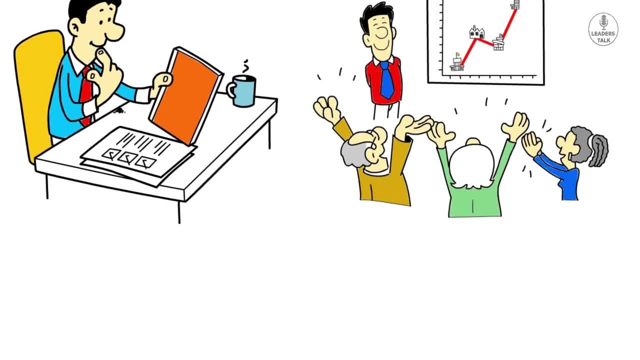 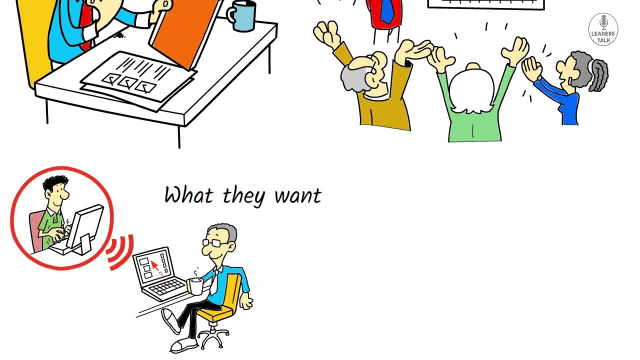 products and services. Data analysis can provide businesses with information about how customers interact with their products or services, what they like and dislike and what they are willing to pay for. For example, a technology company may analyze social media data to find out what their 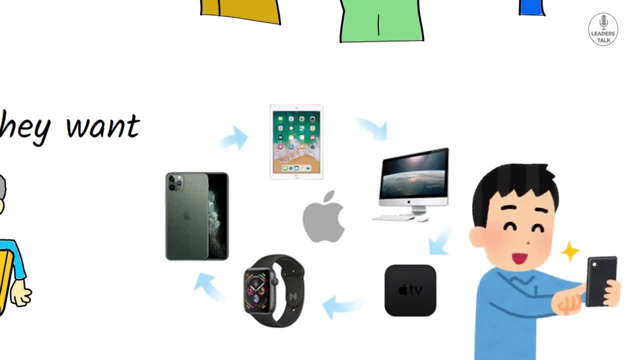 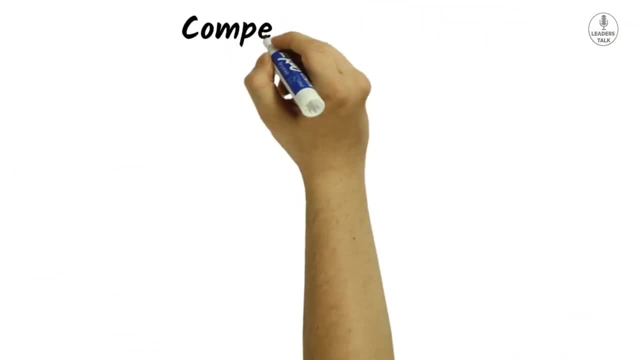 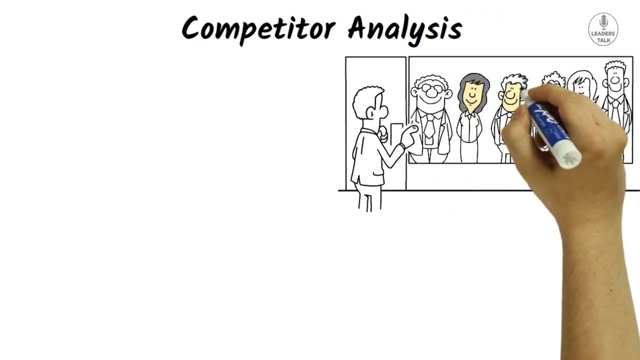 customers are looking for in a new smartphone. This information can then be used to develop a new product that meets those needs. Another type of market research is competitor analysis. This involves gathering information about the competition, such as their products and services, pricing and marketing strategies. Competitor analysis can help businesses identify areas. 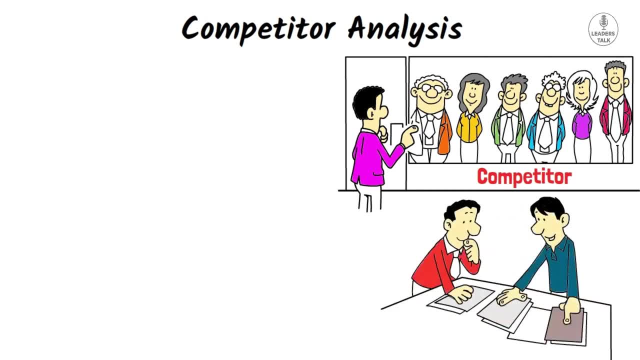 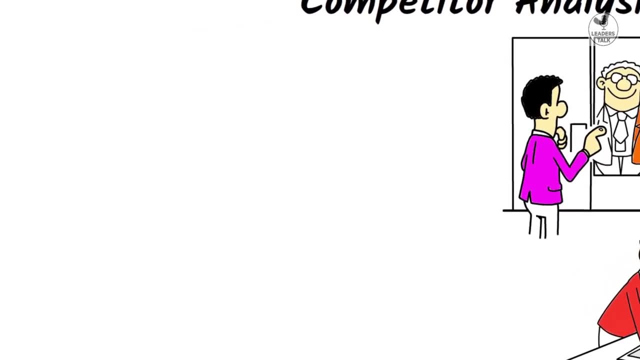 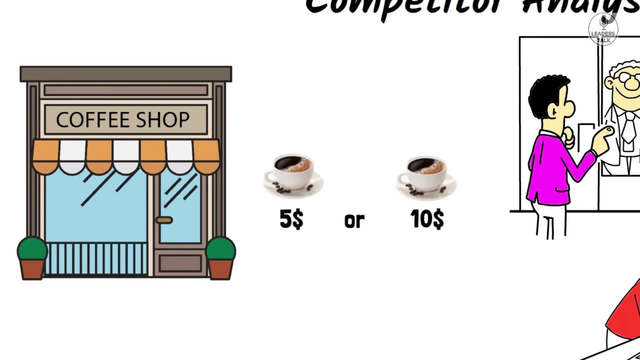 where they can differentiate themselves and gain a competitive advantage. By understanding what their competitors are doing, businesses can identify gaps in the market and develop strategies to fill those gaps. For example, a coffee shop may analyze the menu offerings and pricing of other coffee shops in the area to determine what types of products and pricing strategies are most. 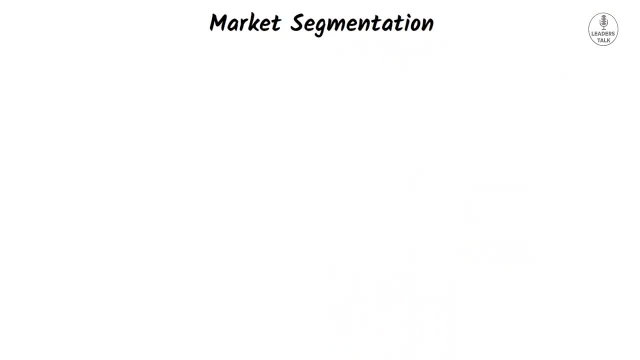 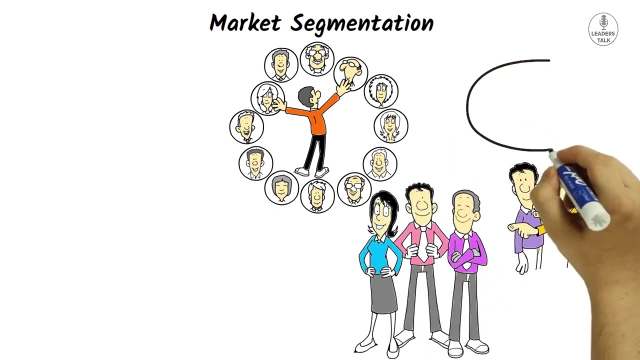 effective Market segmentation is another important element of market research. It involves dividing a market into smaller groups of consumers with similar needs and characteristics. By understanding the different segments of a target audience, businesses can create targeted marketing campaigns and develop products and services that meet the specific needs of each segment. 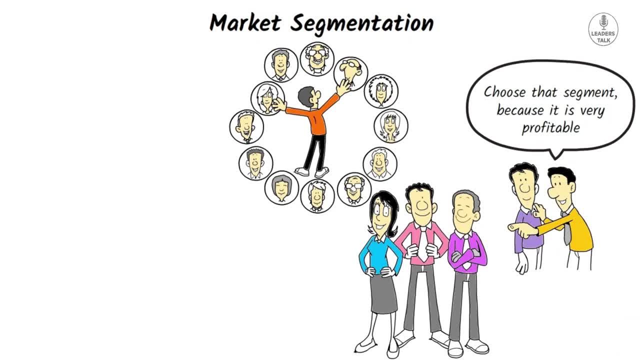 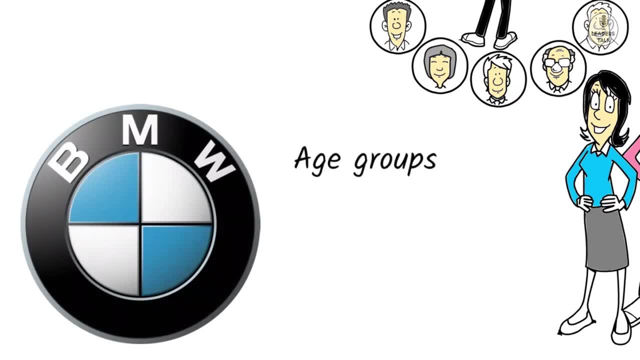 Market segmentation can help businesses identify which segments are most profitable and where they should focus their marketing efforts. For example, a car manufacturer may segment its target audience into different age groups, income levels and lifestyles to develop vehicles that meet the needs of each segment. 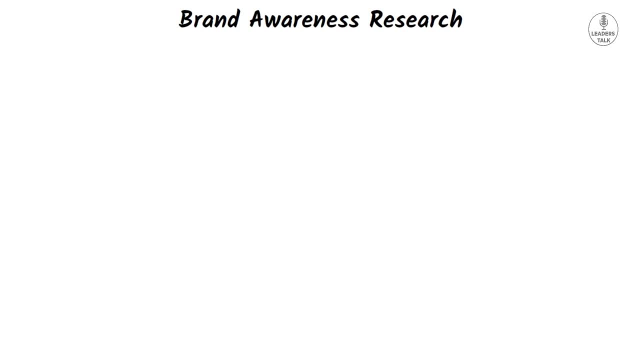 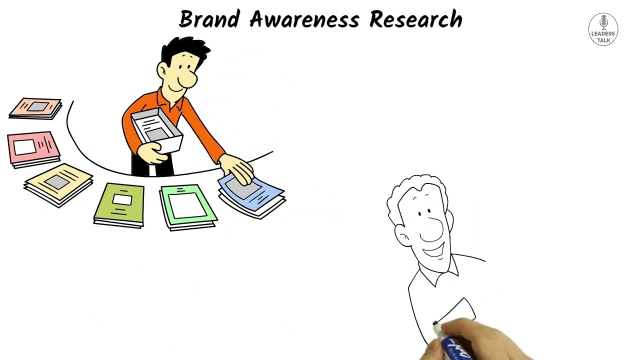 Brand awareness research is also important for businesses. It involves gathering information about how well-known a brand is and what associations people have with the brand. This information can be used to develop marketing strategies that improve brand recognition and build brand loyalty. Brand awareness research can help. 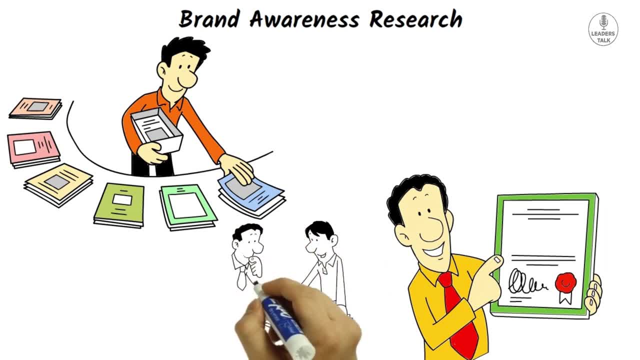 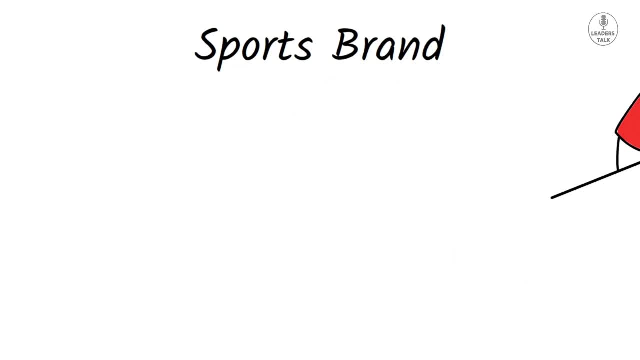 businesses understand how their brand is perceived by their target audience and identify areas where they need to improve their brand image. For example, a sports brand may conduct brand awareness research to understand how well-known their brand is among different age groups and what associations people have with the brand. This information can be used. 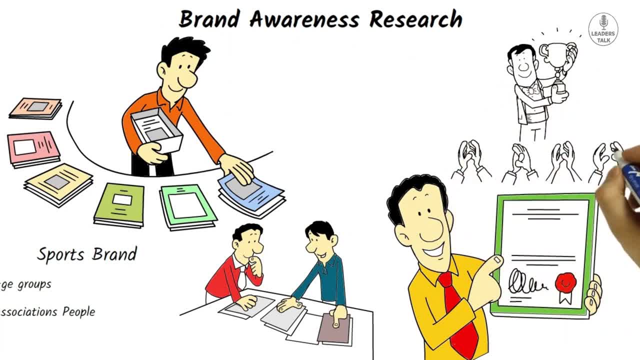 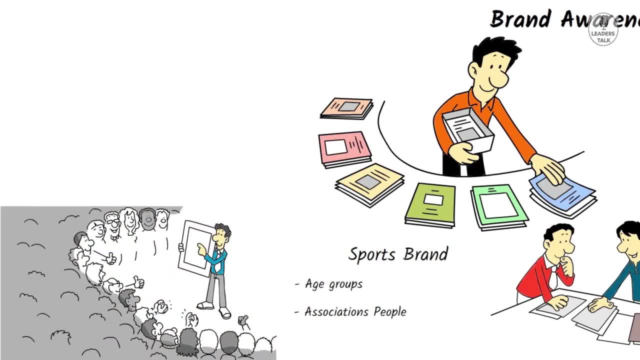 to develop marketing strategies that improve brand recognition and build brand loyalty. Brand awareness research can help businesses understand how their brand is perceived by their target audience and identify areas where they need to improve their brand image. For example, a sports brand may conduct brand awareness research to understand how well-known 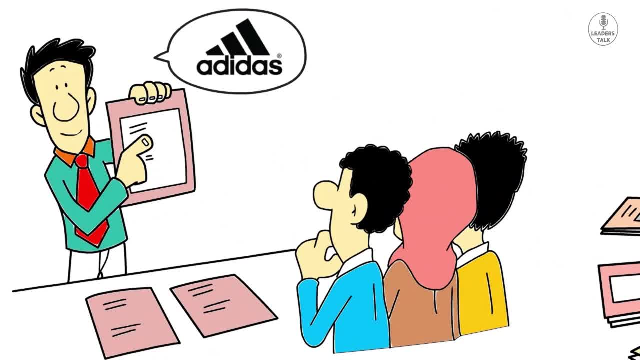 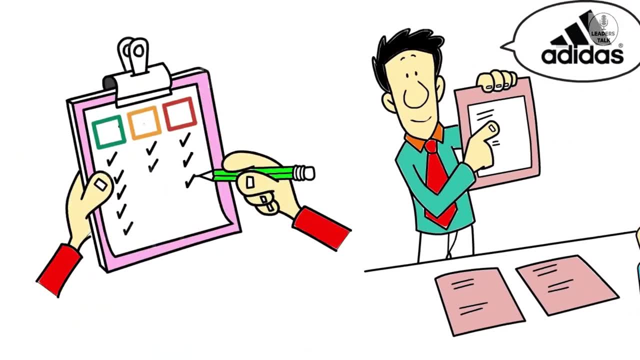 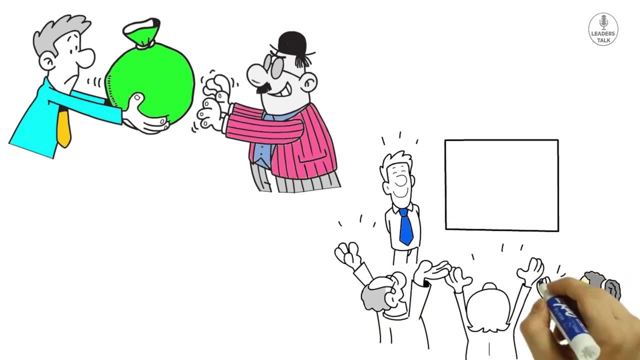 their brand is among different age groups and what people associate with their brand. Based on this information, they can develop marketing campaigns that target specific age groups and emphasize different aspects of their brand. Market research can be time-consuming and expensive, but it is a necessary investment for any business that wants to succeed in. 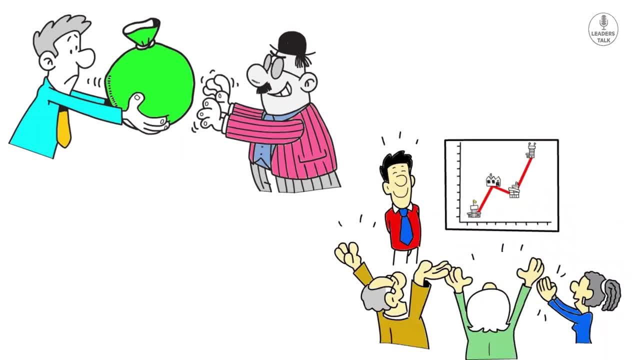 today's competitive market. It helps businesses make informed decisions, reduces the risk of failure and increases the chances of success. By using the right market research methods and analyzing the data correctly, businesses can gain a deeper understanding of their customers and the market in which they operate.